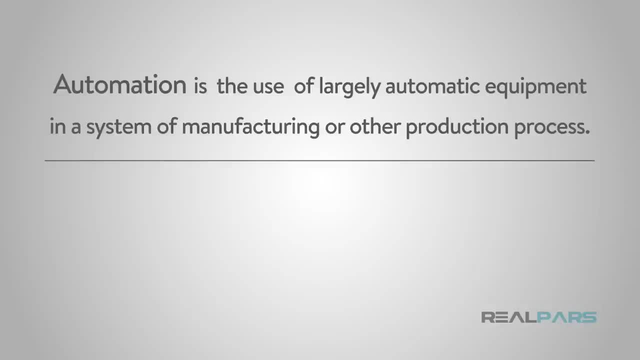 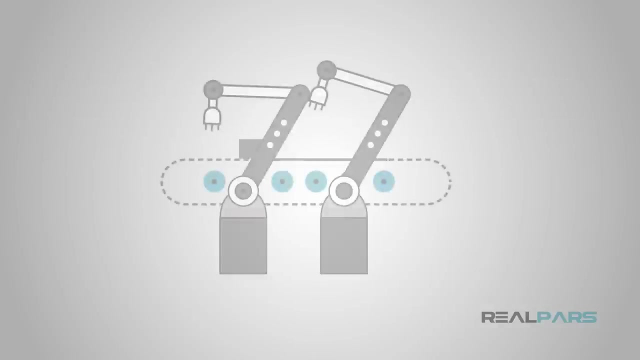 in a system of manufacturing or other production process. This typically includes the use of PLCs, sensors, robots and motors, among many other things. depending on the automated process, Almost any process can become automated. It can save time and money to automate. 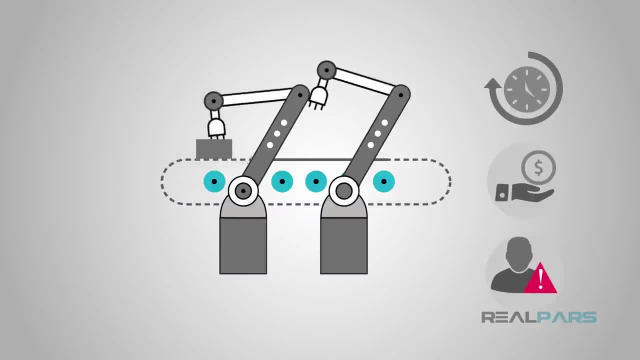 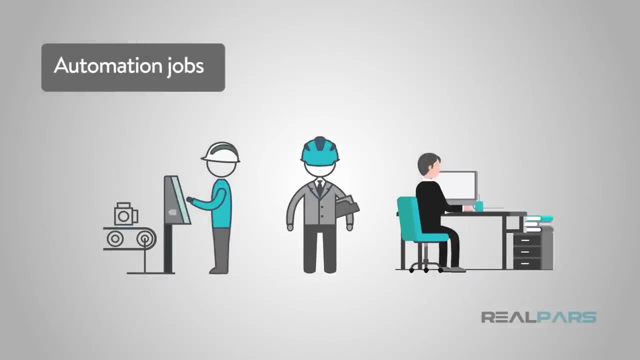 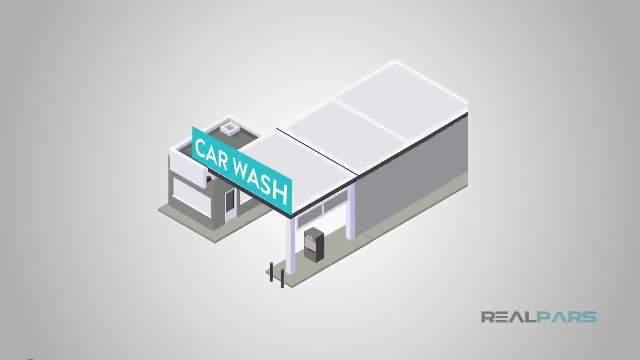 an industrial process. It also helps eliminate human error. Another upside is that the use of automation creates many high-paying careers for maintenance workers, engineers and programmers. A simple everyday example of automation would be an ordinary pull-in and park automatic car wash. 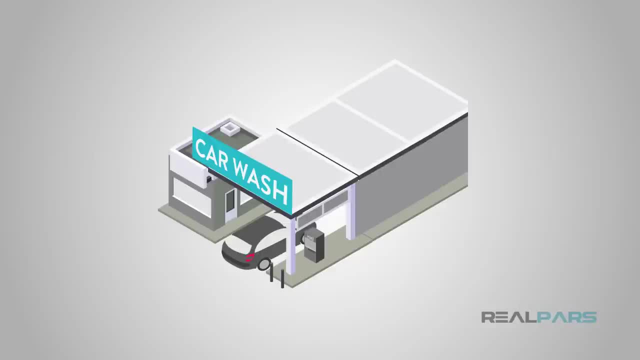 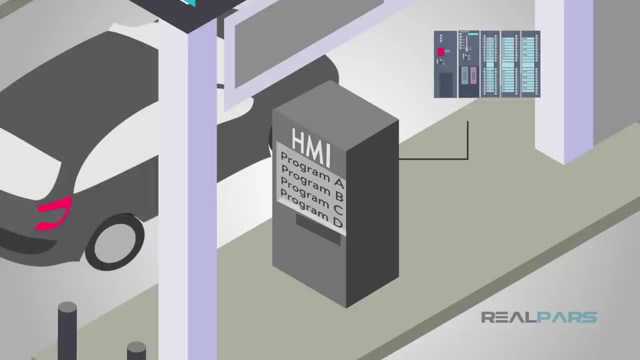 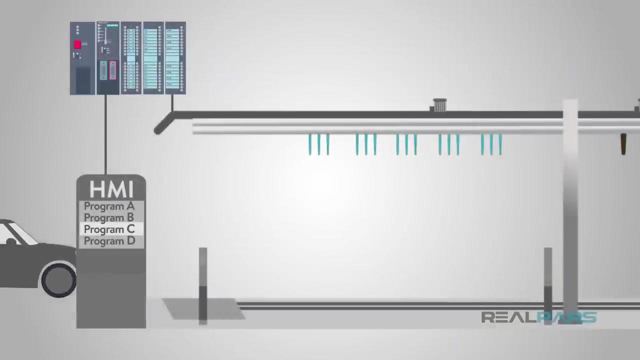 If we break it down step by step, it should help you understand how it works. Once you select your wash, that input will run a certain program on the controller. Next you drive forward until a sensor is flagged, starting the wash cycle. 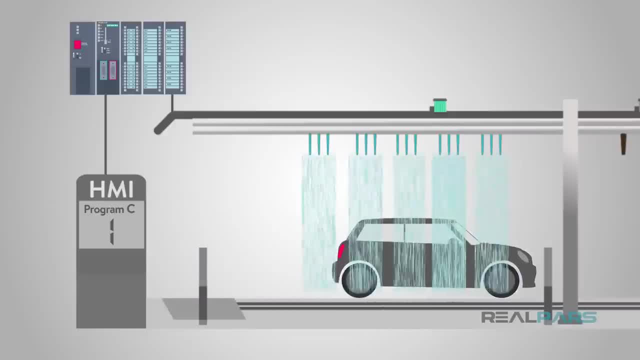 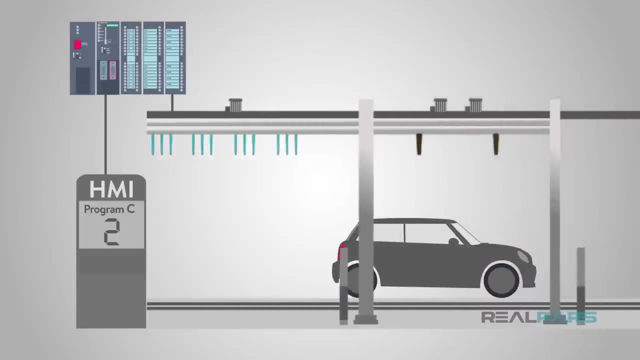 and another sensor tells the driver when to stop. From there, the wash will continue through the cycle that the controller is running. In a typical car wash, the driver is the one who will stop The nozzle spraying the water and chemicals will travel alongside a vehicle. 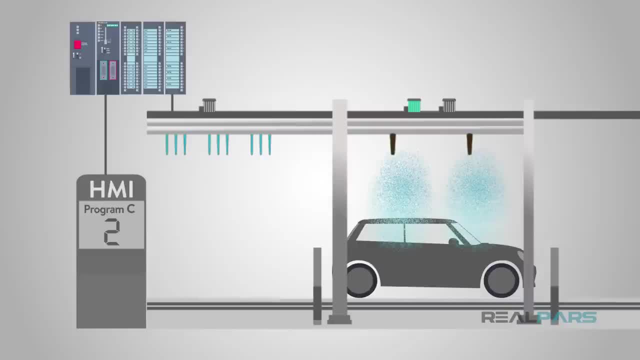 and a sensor will detect when it is past the vehicle. This saves time, water and chemicals by controlling when the nozzle spray, as well as serves as an input to advance to the next step of the wash. Once the car is sprayed, the program tells the wash to spray the next chemical. 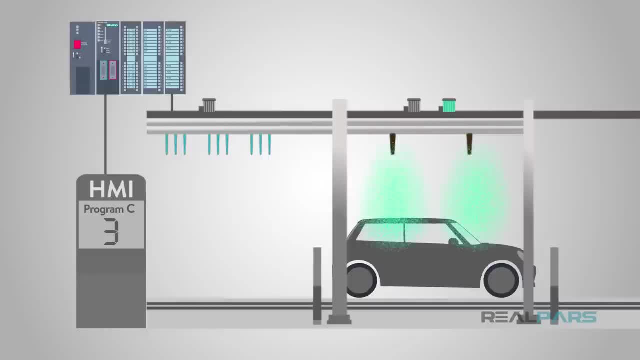 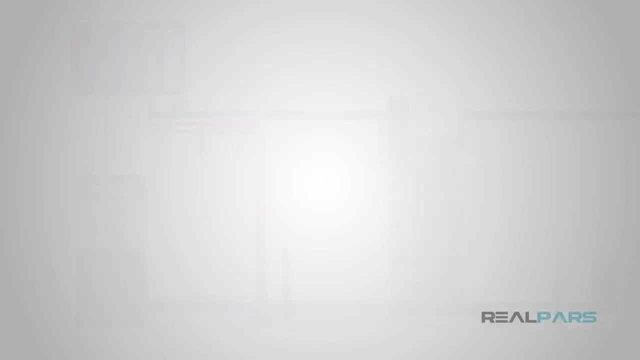 This is done by the controller turning on the nozzle spray on and off each pump as it's needed. The controller then runs through the rest of the cycle and wash that was selected in the beginning. Once all steps have been completed, the driver will be signaled to pull out of the wash. 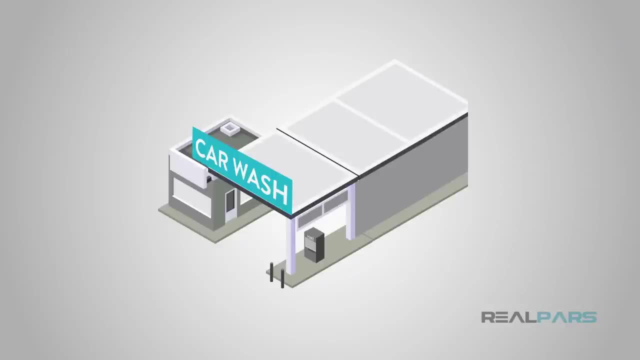 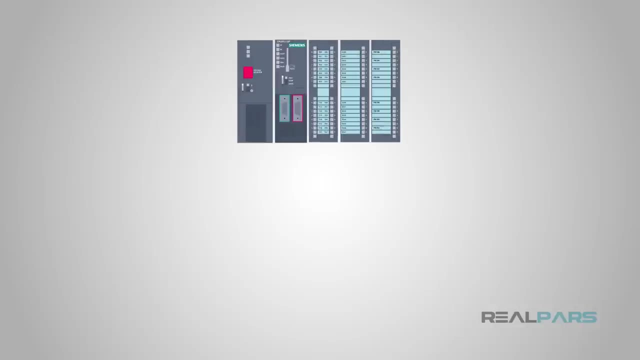 Essentially, the only human intervention in the process is the driver selecting what wash they want. Industrial automation works exactly the same way. Each industrial process needs to be started by some sort of input. That input can be a sensor, push-button switch, among many other possibilities. 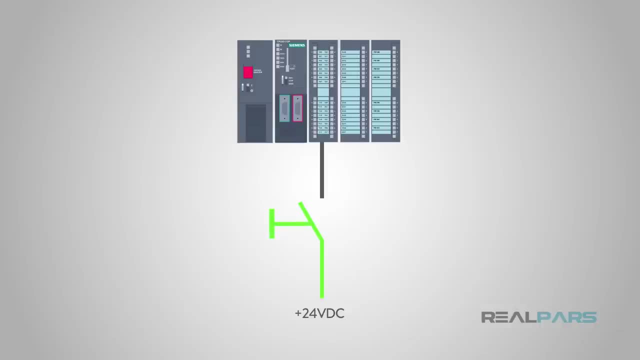 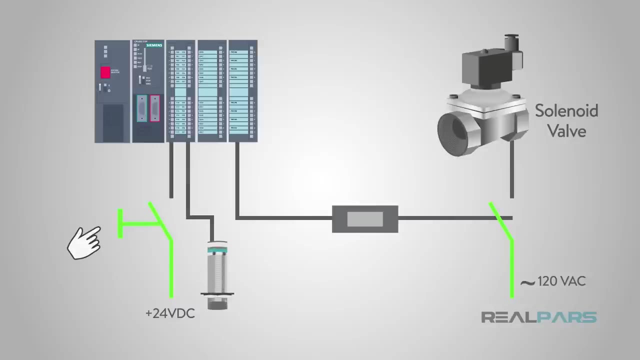 Typically, a person will start the process with one of these input devices, or it could be a sensor that detects an object automatically. Those inputs will go to a PLC or a sensor that detects an object automatically. These inputs will go to a PLC or a sensor that detects an object automatically. 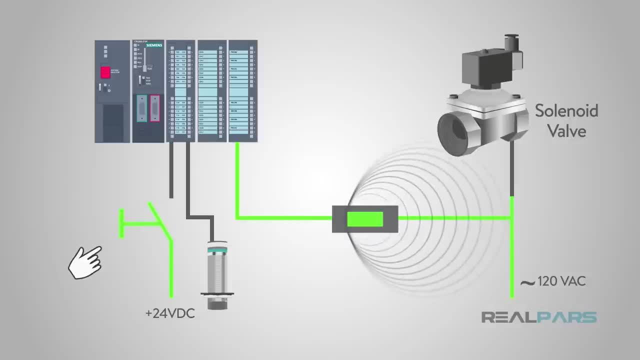 These inputs will go to a PLC, which will then make decisions based on how it was programmed. The PLC will then activate whatever output the program says to run. An output can be anything that does work, such as a motor, solenoid heater or a light. 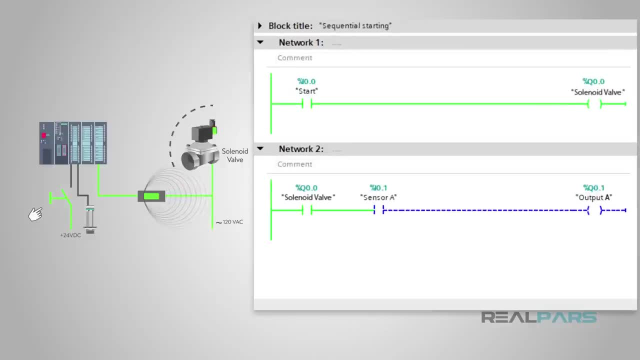 In an automated process, that output will typically be programmed as an input to the PLC and combined with other input devices or programming to keep the process running. With this programming it can act like a chain reaction, with one output device starting before the next is allowed to run. 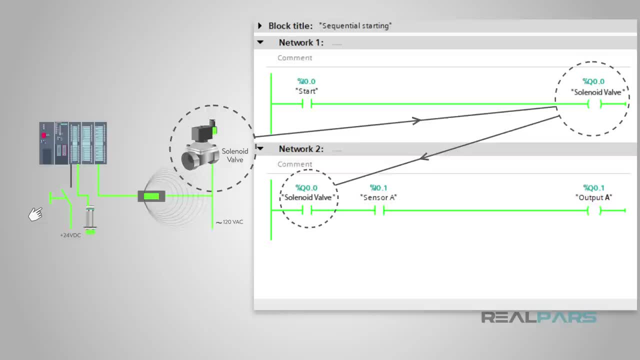 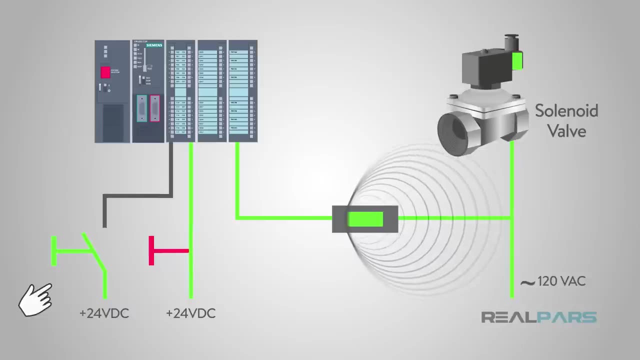 This is also called sequential starting. Automation has to have many aspects working together in order to function properly. An automated process will continue its cycle until it receives a stop signal. That can come from a physical input such as a stop button or sensor, or something programmed like a timer. 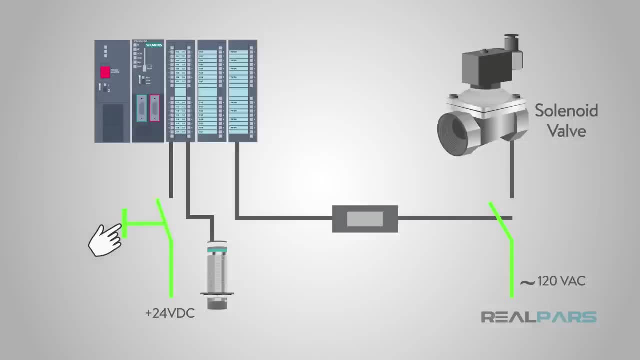 Let's look back at what we now know. Automation is an automatic process typically controlled by computers and sensors. There is usually very little human intervention. Input devices such as sensors and sensors and switches will work with a controller or PLC to activate output devices like motors or other machinery.